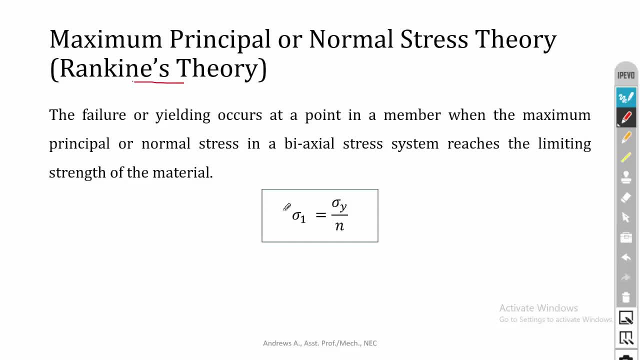 So, since we are dealing with biaxial stress system, there will be two stress components, that is, x direction and y direction. So by combining the x and y direction, we are going to calculate the normal stress, that is, maximum principle stress. So when the maximum principle 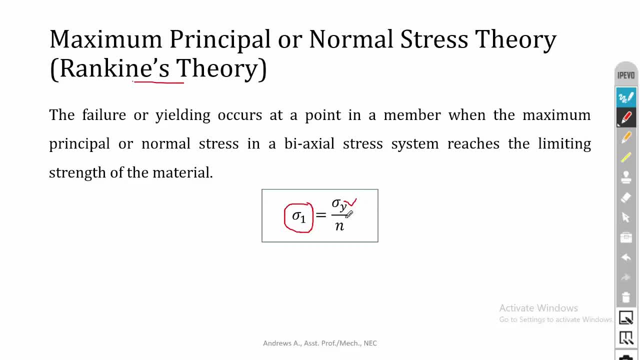 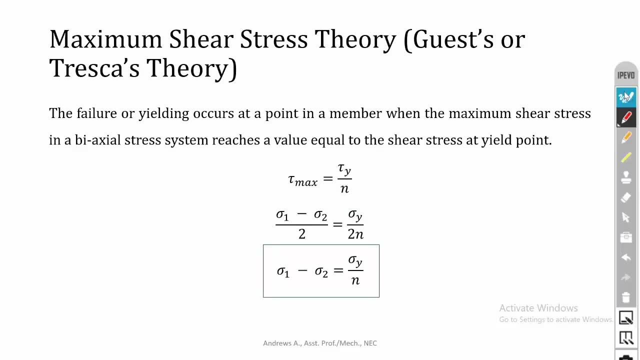 stress is above the yield strength, then the material will break. However, n is the factor of safety. So for all the materials the n should be minimum of 1.. Then the next theory is maximum shear stress theory. So this theory is called as Guest theory, or Tresca's theory. According to this, 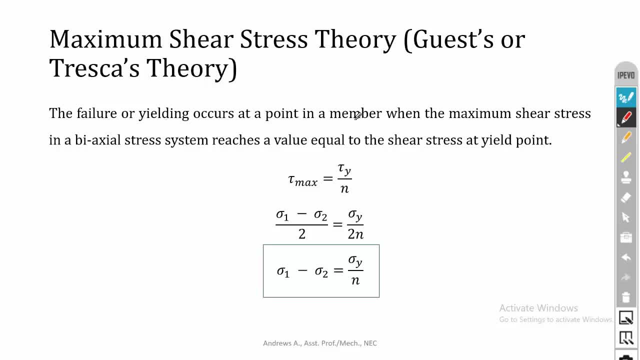 theory the failure or yielding occurs at a point in a member when the maximum shear stress in a biaxial stress system reaches a value equal to the shear stress at the minimum yield point. So all the materials have some yield stress values. So when we apply, 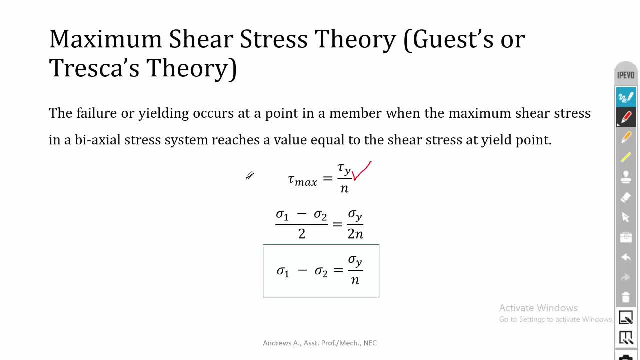 external load on any component. if the maximum stress at any point on the component exceeds the yield strength of the material, that is, shear strength of the material, then the material will break. So the equation is: tau max is equal to tau y divided by n. We know that. tau max is equal to sigma1 minus sigma2 minus ta x. The axial cum tractatebar is possible in any area of the room. So tau x haltonbase will be 對. the rate atnymi is equal toauальная0.0Nuh. 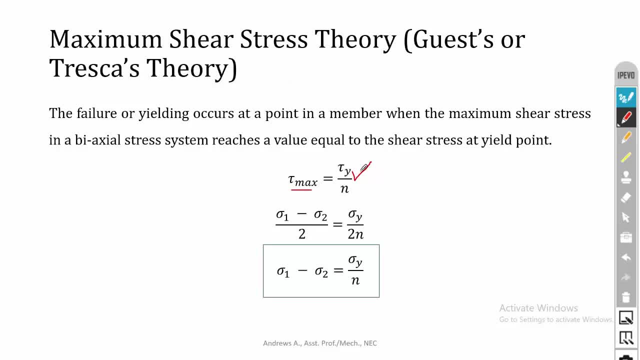 two divided by two, and according to the maximum shear stress theory, tau y is equal to sigma y divided by two. so I am substituting it. tau y is equal to sigma y divided by two and n, so two, two will get cancelled. finally, we will get sigma one minus sigma two, that is equal. 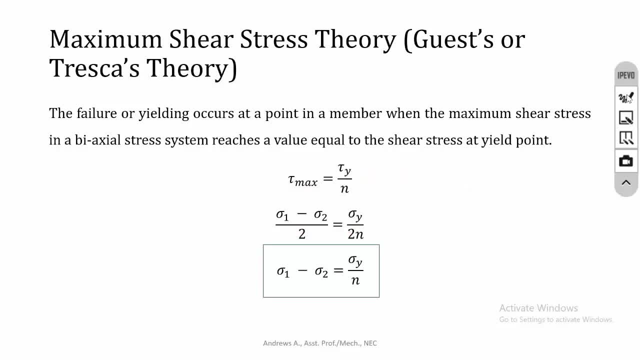 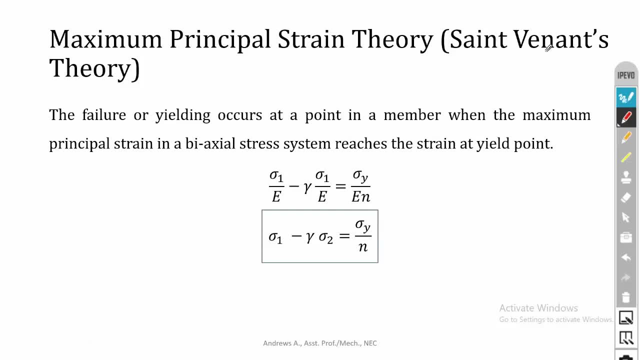 to sigma y divided by n. The next theory is maximum principle strain theory or St Venant's theory. So according to this theory, the failure or yielding occurs at a point in a member when the maximum principle strain in a biaxial stress system reaches the strain at yield. 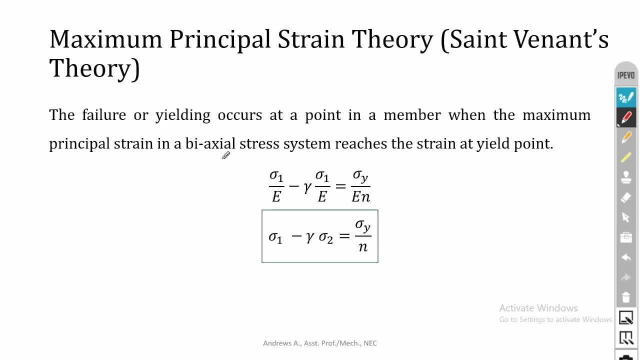 point. So when the external loading is applied, if the maximum principle strain on the component exceeds the strain at the yield point, Then the material becomes unstable, will break. We know that strain is equal to sigma by E, so this is the strain in one direction. 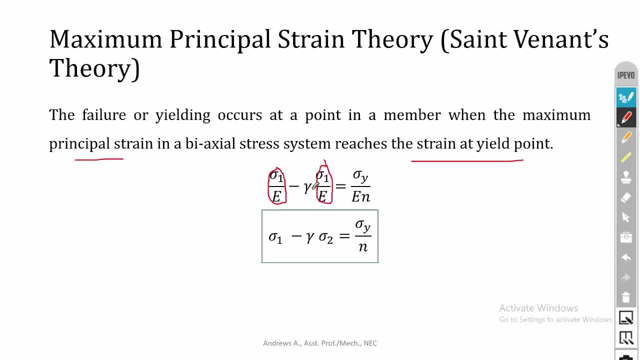 minus gamma into strain in another direction. So this gamma is Poisson ratio, that is lateral strain divided by longitudinal strain. that is equal to sigma y divided by E into n. So E will get cancelled. finally, we will get sigma 1 minus gamma into sigma 2, that is equal to. 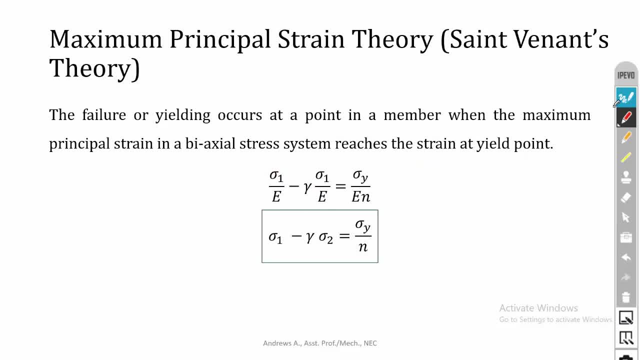 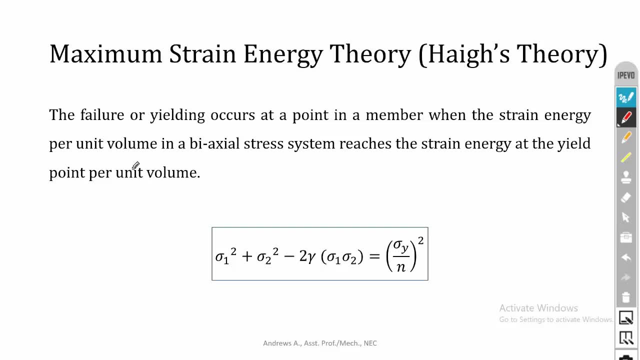 sigma y divided by n. The next theory is maximum strain energy theory or height theory. So according to this theory, the failure occurs at point in the member when the strain energy per unit volume in the biaxial stress system reaches the strain energy at yield point per. 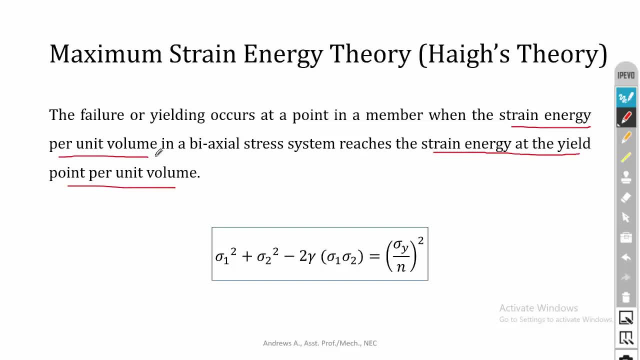 unit volume. When the strain energy per unit volume of at any point on the component exceeds the strain energy solution, it grades to be equal. So that is, when the strain energy and the strain energy at the yield point, then the material will break. So this is the equation for maximum strain energy theory: sigma1 square plus sigma2 square. 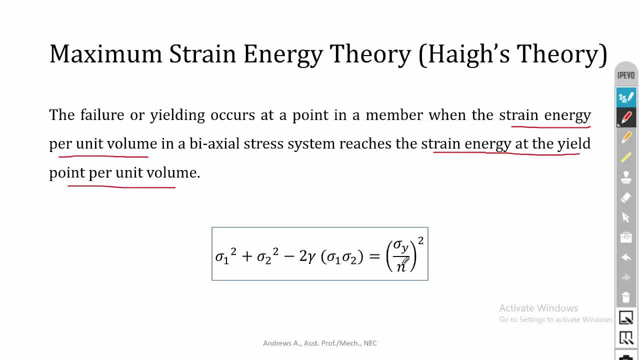 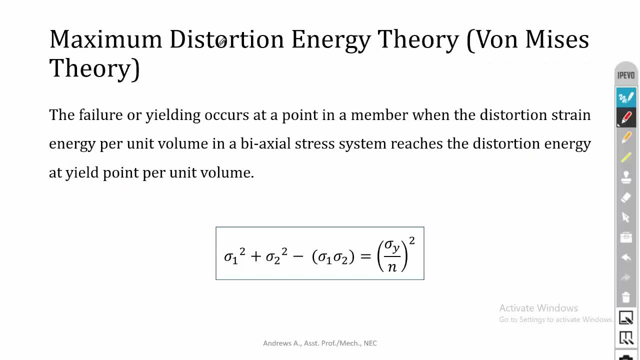 minus 2, gamma, sigma1, sigma2, that is equal to sigma y divided by n, the whole square. Then the last theory is maximum distortion energy theory, or Von Mises theory. So this theory is mostly used in our mechanical applications. The failure or yielding occurs at a point in a member when the distortion strain energy. 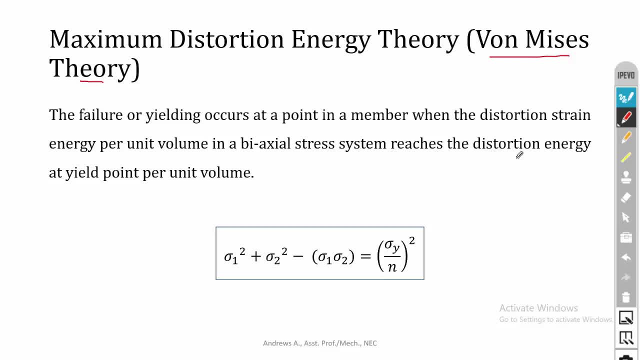 per unit volume in a biaxial stress system reaches the distortion energy at yield point per unit volume. So when the distortion energy per unit volume exceeds the distortion energy at yield point, then the system will break. So this is the equation. This is the equation for maximum distortion energy theory: sigma1 square plus sigma2 square. 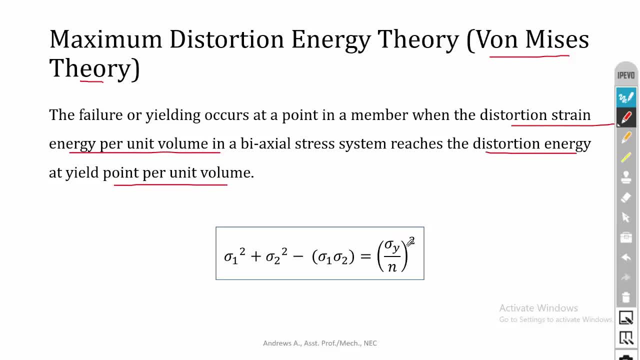 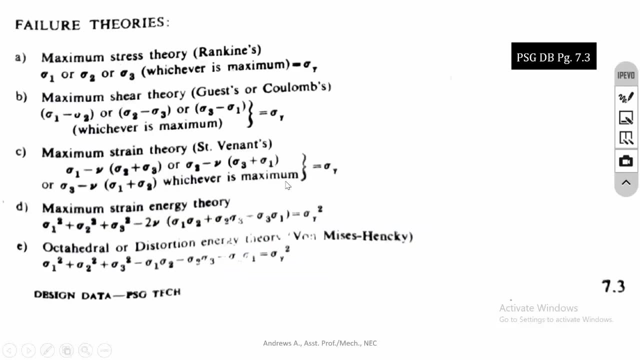 minus sigma1, sigma2, that is equal to sigma y divided by n, the whole square. So this is all about the theories of failure. So by using these theories of failure, we can identify the condition at which any material will fail under the application of external load. 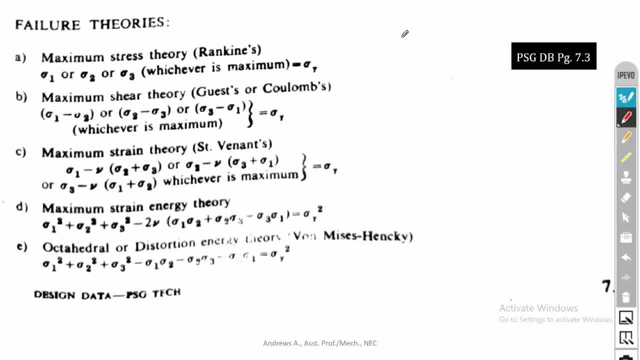 So these equations are there in your data book. I have uploaded the scanned cards. I have put the scanned copy of the data book for your reference. So in that if you take page number 7.3, then these are all the failure theories. 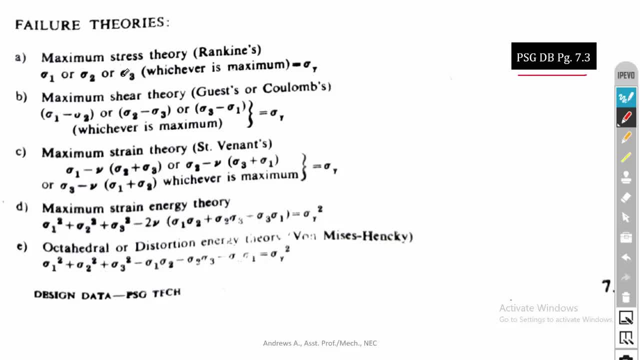 So here, actually, there are three stress components, are there? This is actually for tri-axial stress. Since we are dealing with biaxial stress, then we can put: sigma3 is equal to 0.. So here, sigma1 or sigma2, whichever is maximum, is equal to sigma y divided by n. 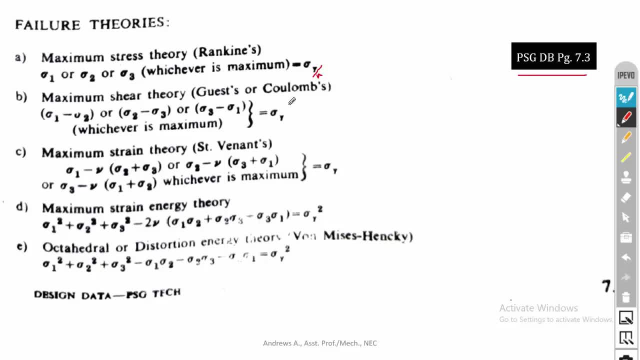 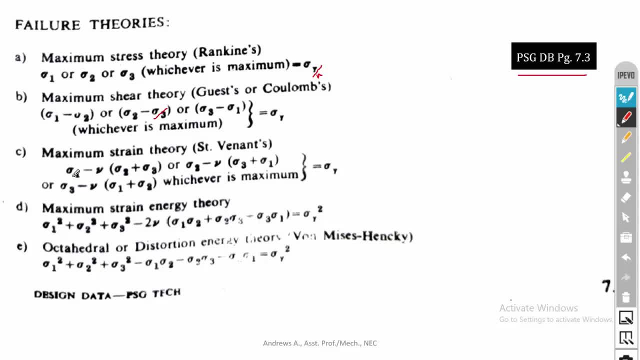 So sigma1 minus sigma2 is equal to sigma y. Then in the maximum strain theory it is sigma1 minus gamma into sigma2.. Since sigma3 is 0, we will get sigma1 minus gamma. sigma2 is equal to sigma y. Then in the maximum strain theory put sigma3 is equal to 0. 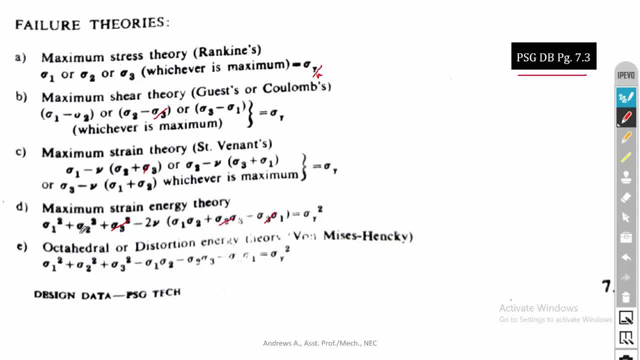 So this is 0.. This is 0 and this is also 0.. So you will get sigma1 square plus sigma2 square minus 2.5.. So this is 0.. Double 2 is equal to 0.. So this is 0.. 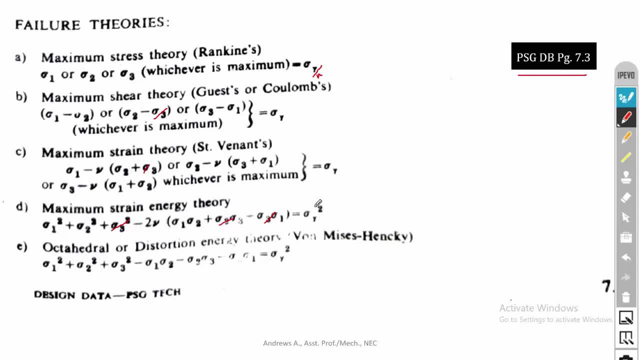 Simple thing. This is 1.. Now, what will be our answer to sigma1?? We will have 0. there We are going to calculate sigma of equal to 0. So sigma1 minus sigma2 is equal to sigma1 plus sigma2 is equal to sigmay divided by n. 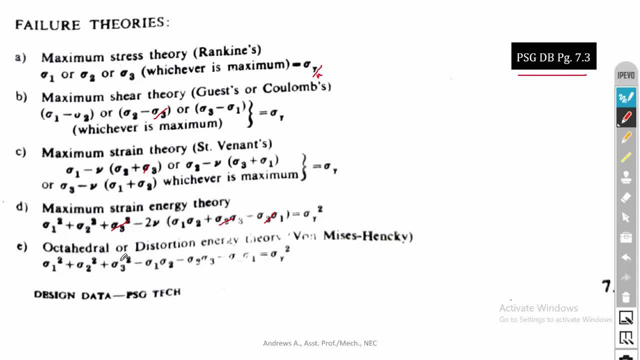 for the whole square. Don't forget to put the next factor of safety. And in the 1-mices theory we put: sigma3 is equal to zero, So 0 zero, 0, 0, zero 0 and we will get sigma1 square plus sigma2 square minus li제1. 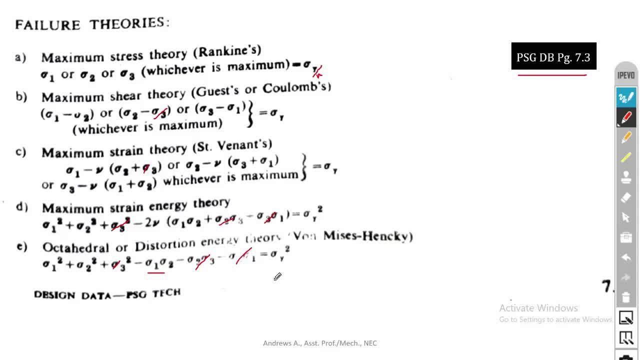 籵환. uma1 sigma2 is equal to sigma y, divided by n is equal to whole square. Okay, so you don't need to memorize these equations. All these formulas are available for you to apply. are available in the data book, page number 7.3.. 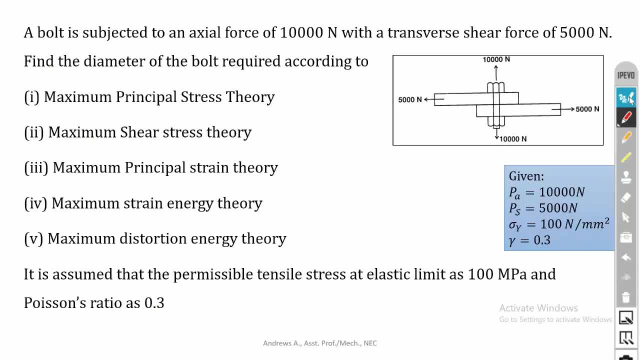 With this we will move into the problem. I am going to tell you a simple problem. So in this problem we are going to use all the 5 theories. A bolt is subjected to an axial force of 10,000 N with a transverse shear force of 5,000 N. 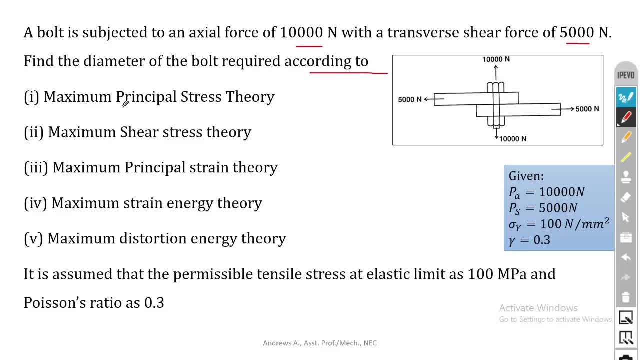 Find the diameter of the bolt required according to maximum principal stress theory, maximum shear stress theory, maximum principal strain theory, maximum strain energy theory and, finally, maximum distortion energy theory. It is assumed that the permissible tensile stress at elastic limit as 100 MPa, that is. 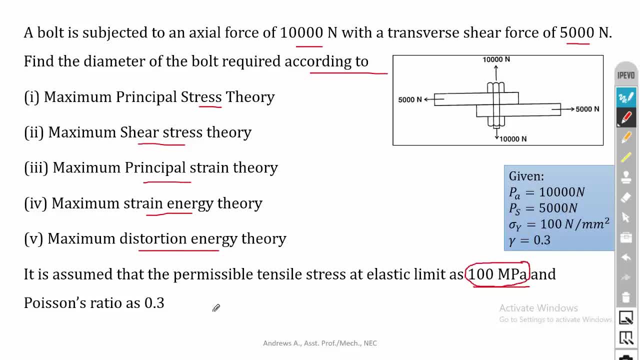 nothing but sigma y is equal to 100 N per mm square And Poisson ratio as 0.1.. So this is the given diagram. So you can see the drawing. This is actually the bolt. So this bolt is subjected to an axial tensile load of 10,000 N. 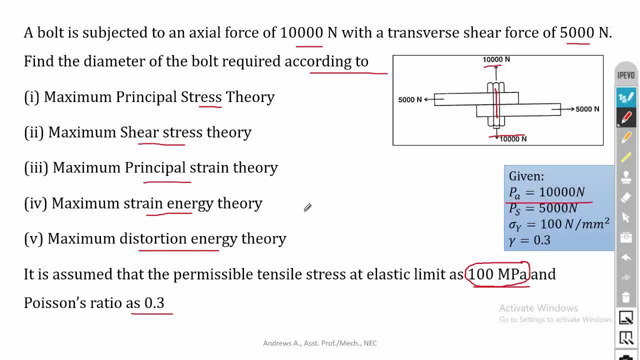 So the first load is axial load, Pa is equal to 10,000 N. Then the secondary load is a transverse shear load. that is actually direct shear. So if the two forces are acting like this, then the material will fail at this location. so this is direct shear. 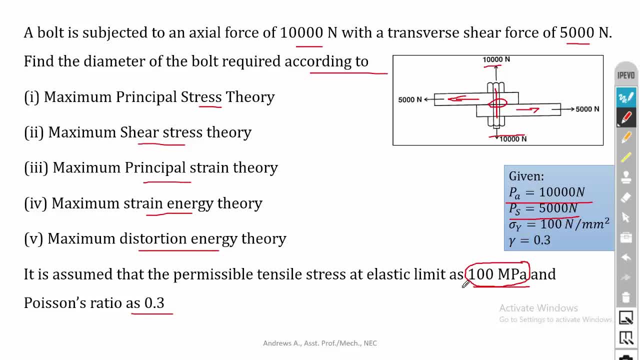 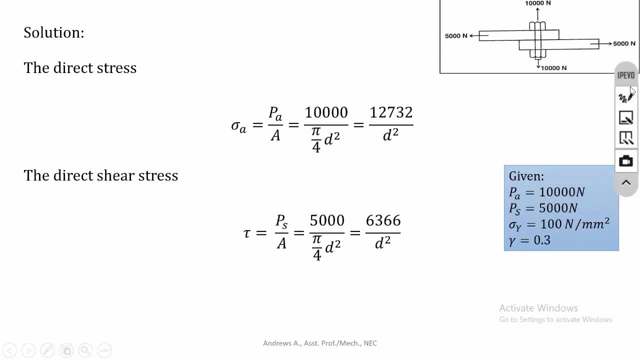 So Ps is equal to 5000 N. Then sigma y is given, it is 100 N per mm square. and finally the Poisson ratio is given: it is 0.3.. There is no unit for Poisson ratio, So in all the theories we are going to use sigma 1 and sigma 2.. 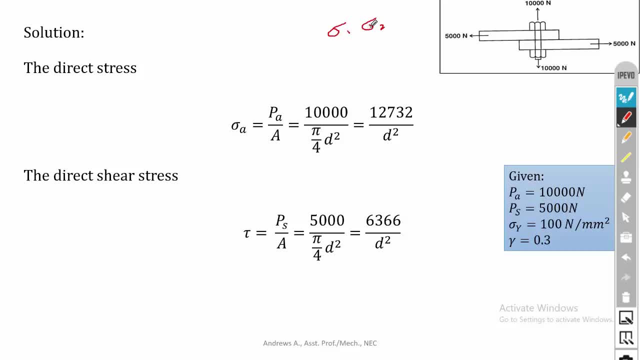 So first step, we have to calculate The maximum and minimum principle stress. So to calculate the maximum and minimum principle stress, first we should calculate the axial stress and the direct shear stress because of these two loads. So this 10,000 N will create an axial stress and this 5000 N will create a direct shear. 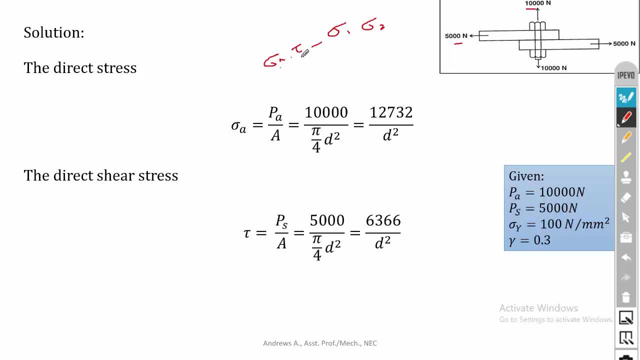 stress. So first we have to calculate the axial stress and the direct shear stress. Then, by using these two stresses, we can calculate the maximum and minimum principle stress. So we will start with the direct stress first. So we know that the equation for axial stress is sigma a is equal to pa divided by a. 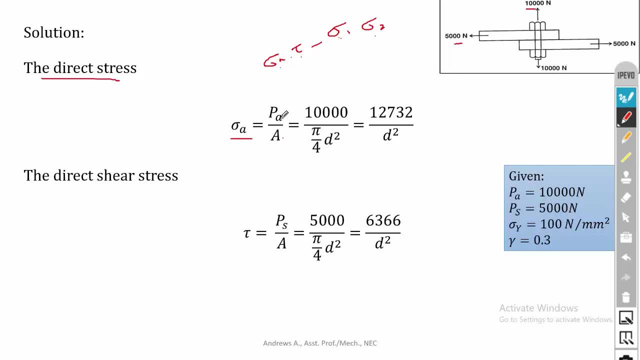 So since it is a bolt, then the cross section is circular. So pa- I have substituted. pa is, given it is 10000, and a, since it is circular cross section, it is pi by 4 d square. So if you solve this equation then you will get 12732 divided by d square. 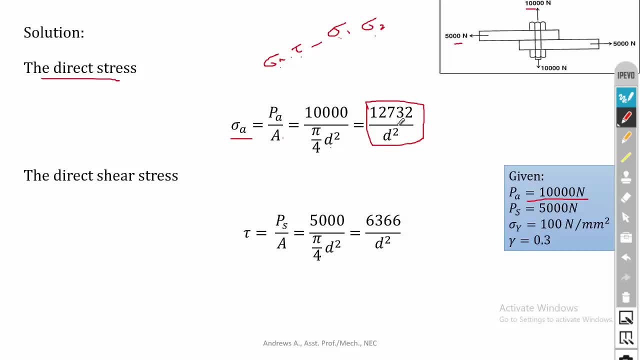 So that we have to calculate the diameter. So in all your values, diameter should be there, d should be there. Then the second one is the direct shear stress. We know that the direct shear stress equation is: tub is equal to ps divided by a. 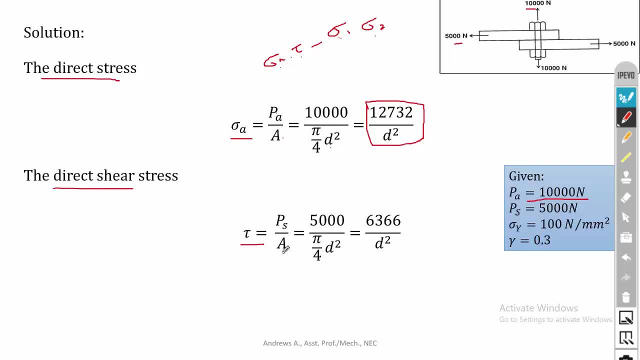 So don't confuse the direct shear stress with the torsional shear stress. So this is direct shear stress. tub is equal to load by area. load is ps. ps- it is given it is 5000 Newton And a. Since it is of circular cross section, then this is the shearing area. 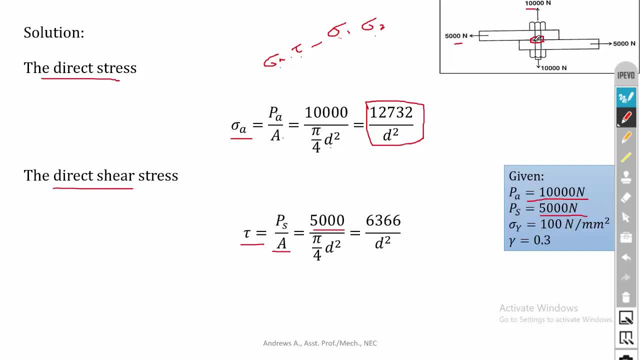 So if we apply the load then it will break at this location. So the shearing area is actually a circular one. So it is pi by 4 d square. So if you solve this, then you will get 6366 divided by d square. 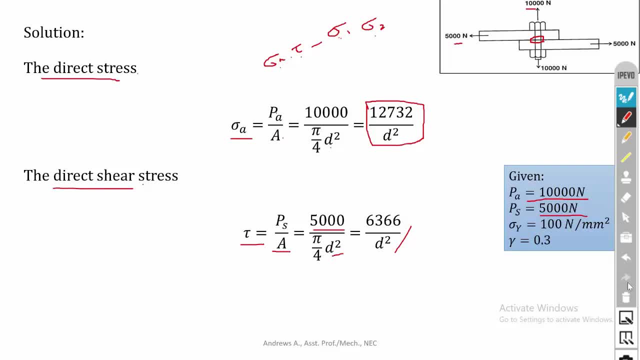 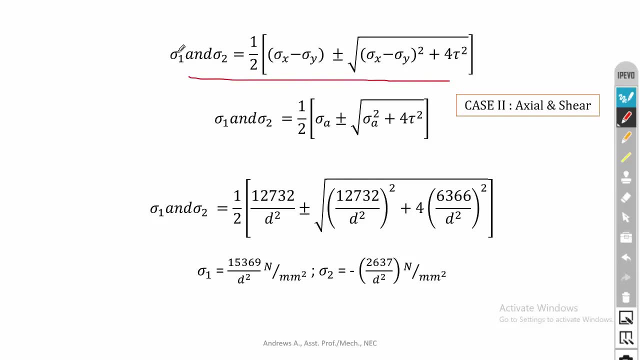 So we have calculated the direct axial stress and direct shear stress. So now we have to calculate the principal stress. So this is the equation. This is the equation to find the principal stress: maximum and minimum principal stress. So according to our consideration, that is, our combined stress cases, this comes under 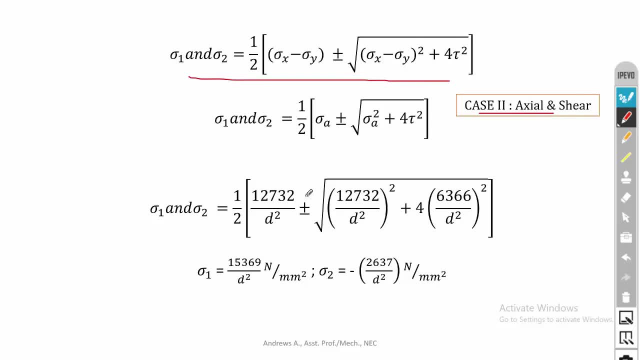 case 2, that is axial and shear. So this is the equation to calculate the maximum and minimum principal stress if we have axial and shear stress. So we have calculated sigma a and tub in the previous step So we can substitute that. I have substituted the value of sigma a. 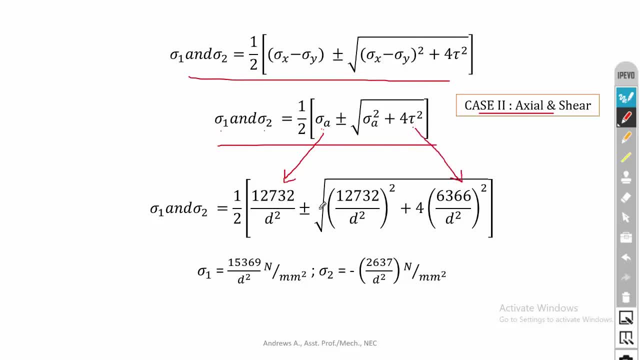 And this is the equation Ok Than, if we put plus, then we will get the maximum principal stress, If we put minus, then we will get the minimum principal stress. So this is the maximum principal stress and minimum principal stress. So now, by having these two principal stress value, we can use the theories of failure. 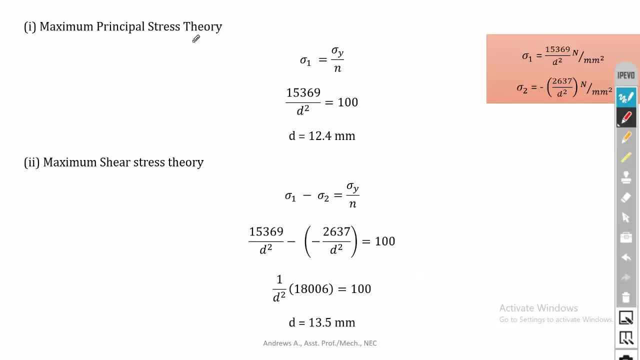 First we will start with maximum principal stress theory prosecuting. So from the data book you can write the equation that is: sigma1 is equal to sigma y divided by n. don't memorize the equations, try to use data books. So sigma1 is equal to sigma y divided by n. 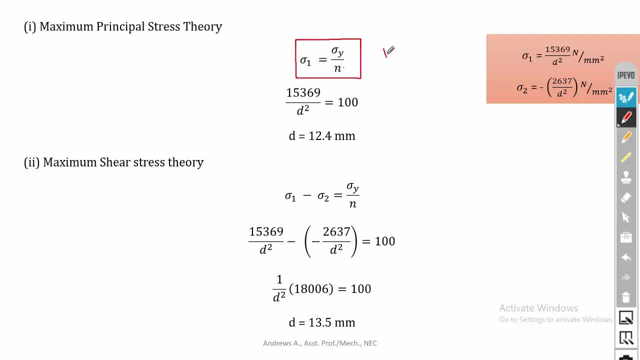 In this problem the factor of safety is not given. so if the factor of safety is not given, we should take a minimum factor of safety of 1, so you have to write: assume n is equal to 1.. So remember that if the factor of safety is not given, we have to assume a minimum factor. 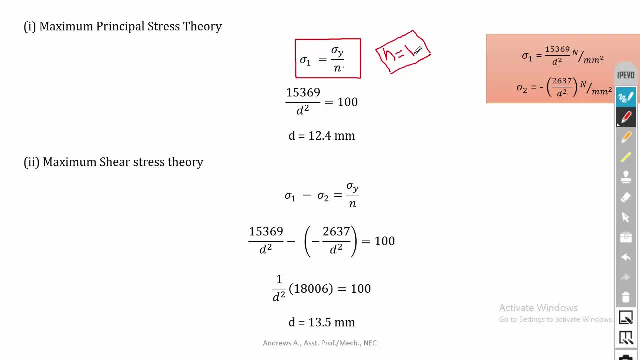 of safety of 1.. So here I have assumed the factor of safety as 1, sigma y is given, so I have substituted it. 100, sigma1. I have calculated in the previous step that is 15369 divided by d square. So if we substitute sigma1 and sigma y, then I can calculate the value for the diameter. 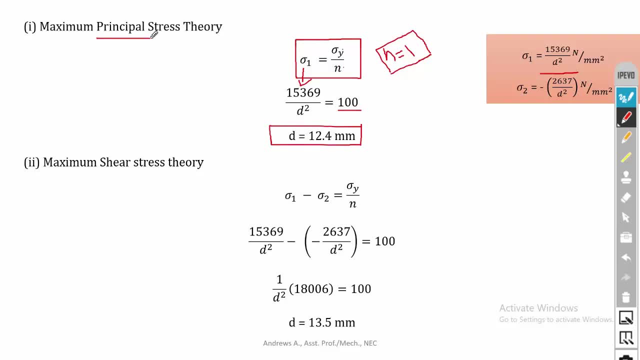 So diameter is equal to 12.4 mm. So this is according to maximum principle. Then coming to the next theory, maximum shear stress theory. So this is the equation: sigma1 minus sigma2 is equal to sigma y divided by n. 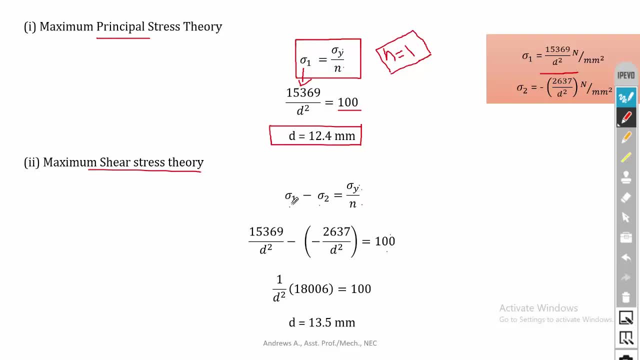 Sigma y value is given. we can substitute that n is equal to 1.. In the previous step we have calculated the value for sigma1, that is maximum principle stress and minimum principle stress. So here the minimum principle stress is in negative. so I have substituted the value. 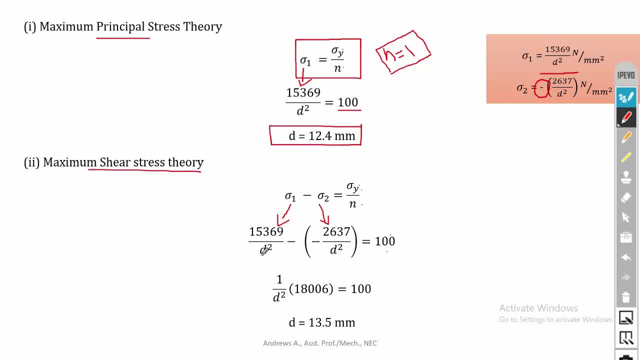 in negative, Then we can take the d square- d square commonly outside, so minus and minus will become plus. take the d square outside, you will get 1 by d square, 1806, that is equal to 100.. So if we solve this then finally we will get: diameter is equal to 13.5 mm. 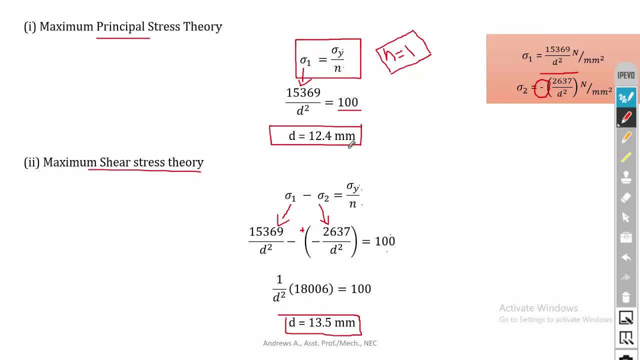 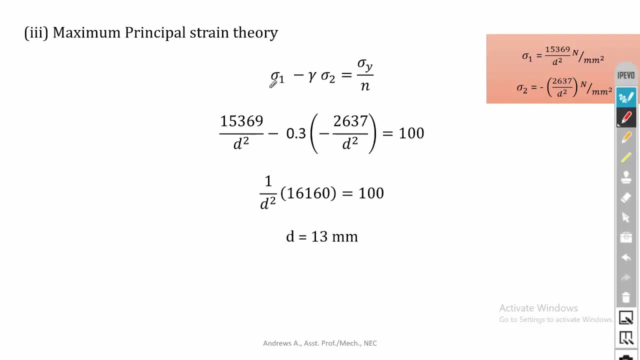 So you can see that. so in the first theory the diameter is 12.4 and here it is 13.5 mm. So there is no much difference in that. Then the next theory is Maximum principle, strain theory. So according to this theory, sigma1 minus gamma sigma2 is equal to sigma y divided by n. 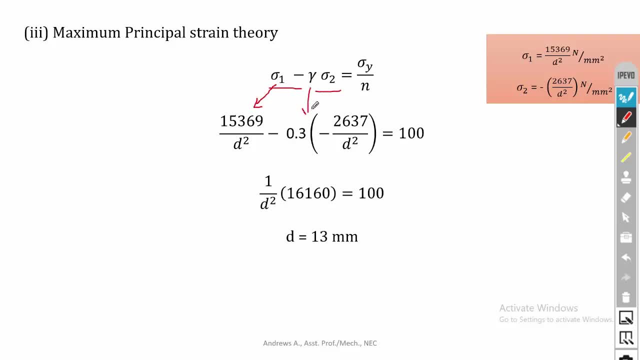 So substitute the value of sigma1, gamma- it is given it is 0.3, then sigma2, sigma y is 100, n is equal to 1.. So take d square commonly outside, then minus and minus you will get plus. so this is your. 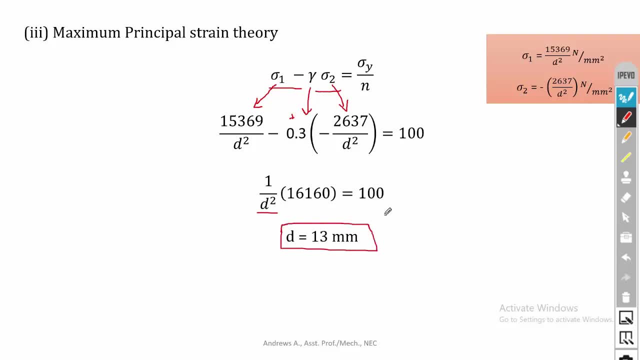 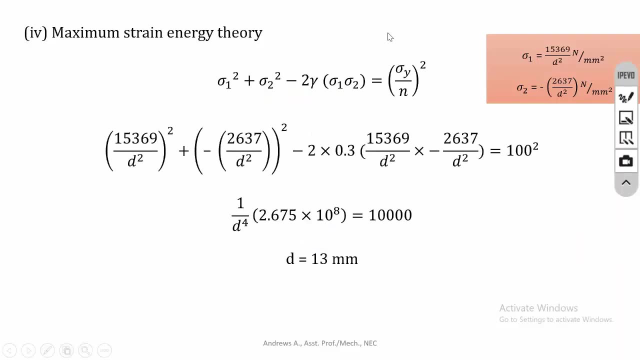 solution. Finally we will get: d is equal to 13 mm. The next one is maximum strain energy theory. So the theory is sigma1 square plus sigma2 square minus 2 gamma sigma1. sigma2 is equal to sigma y divided by n, the whole square. 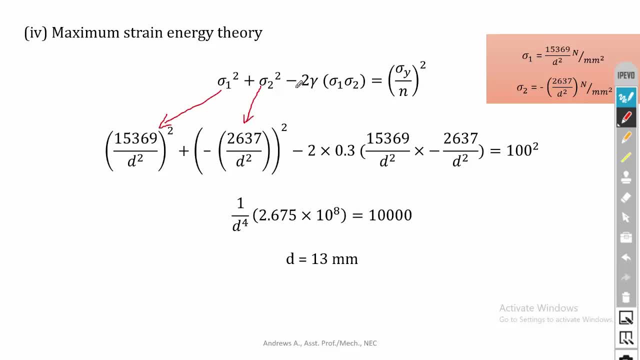 So substitute the value of sigma1, then sigma2.. So remember that here in this equation sigma2 square is there, So it is sigma2, the whole square. That is minus of 2637 by d square, the whole square. So that is very important, whole square. 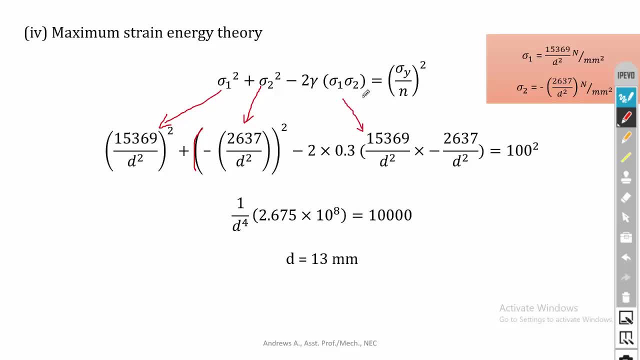 Then minus 2, gamma is 0.3, substitute sigma1, substitute sigma2, and tau y is equal to 100, it is 100 square. So here you will get d square into square d power 4, d power 4, and here also, if you: 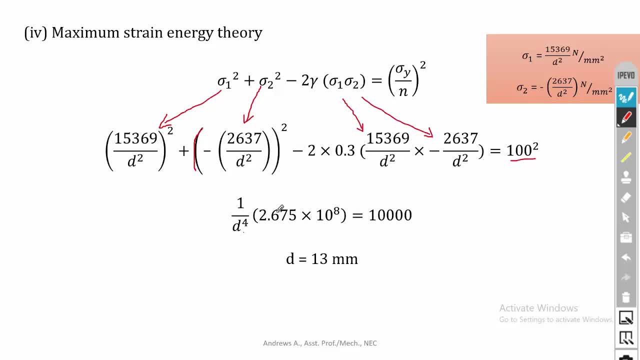 multiply these two, you will get d power 4.. So you can commonly take d power 4 outside and inside. we will get 2.675 into 10 to the power 8.. That is equal to 10000.. So if you solve this equation then finally we will get: d is equal to 13 mm. 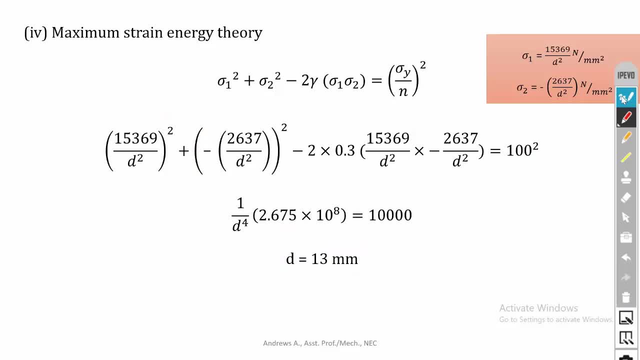 Here also the diameter is 13 mm. Then the next theory is maximum distortion, energy theory. So it is sigma1 square plus sigma2 square minus sigma1. sigma2 is equal to sigma y by n, the whole square. So substitute the value of sigma1, sigma2, then sigma2.. 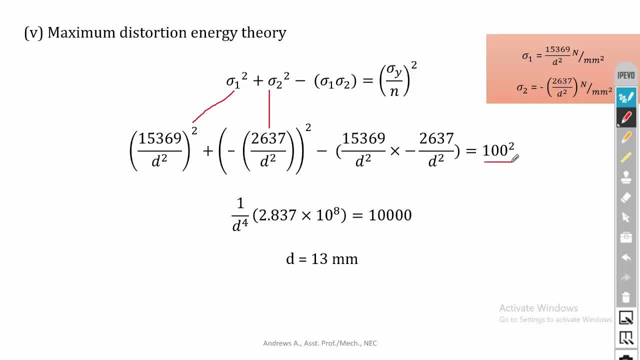 Then sigma1 into sigma2. that is equal to 100 square. Then here you will get d square. I mean d power 4, d power 4, then minus. if you multiply these two then you will get d power 4, take the d power 4 commonly outside, inside that you. 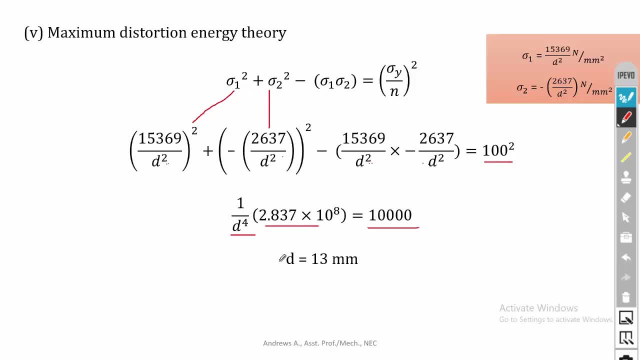 will get 2.837 into 10 to the power 8, that is equal to 10000.. So if you solve this, then finally you will get: d is equal to 13 mm. So here also the diameter is 13 mm. So one thing you have to do is you have to solve this. 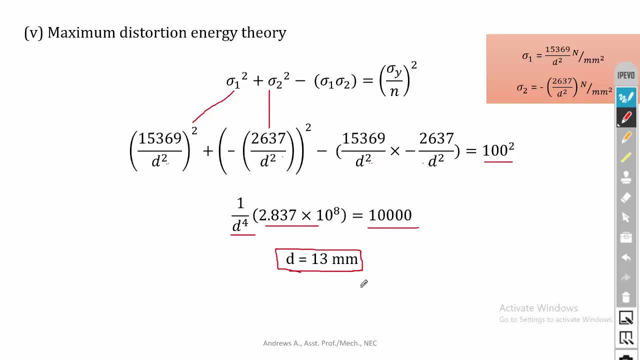 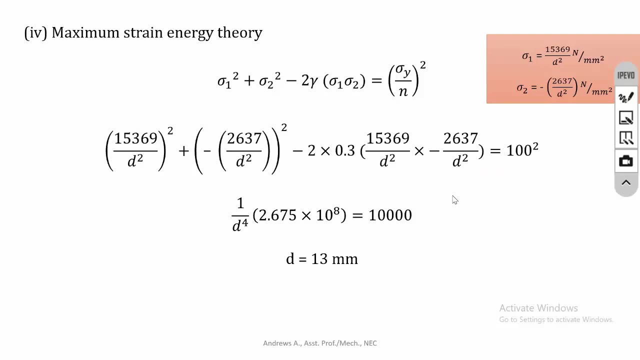 If one thing is very clear, the answer will be uniform in all the theories. So this is how you can verify your solution. So about this problem. first we have to calculate the principal stress equations, That is, principal stress sigma1 and sigma2.. 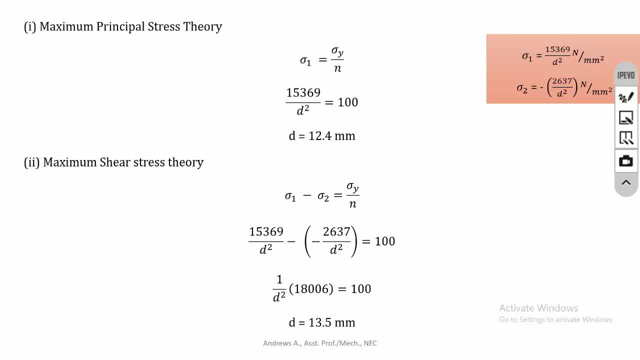 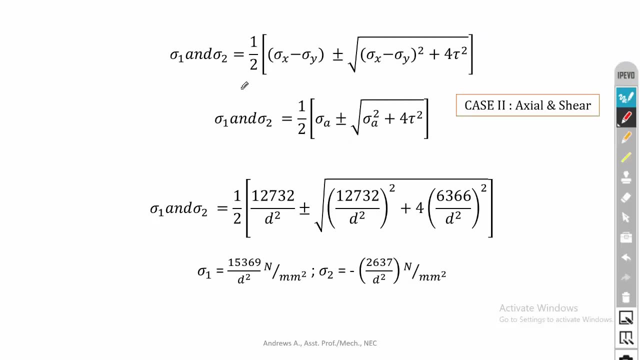 To calculate sigma1 and sigma2, we need the axial stress and direct shear stress. So first we have to calculate the axial stress and the direct shear stress, Then we have to substitute it in the principal stress equations. So after substituting everything in the principal stress equation, then finally you will get the. 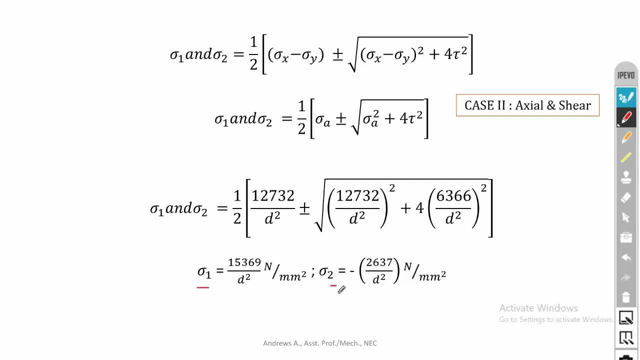 sigma1 and sigma2.. So once if you calculate sigma1 and sigma2, then you can substitute this sigma1 and sigma2 in the theories of failure equations and you can calculate the diameters. So it is important to understand the equations, Okay. 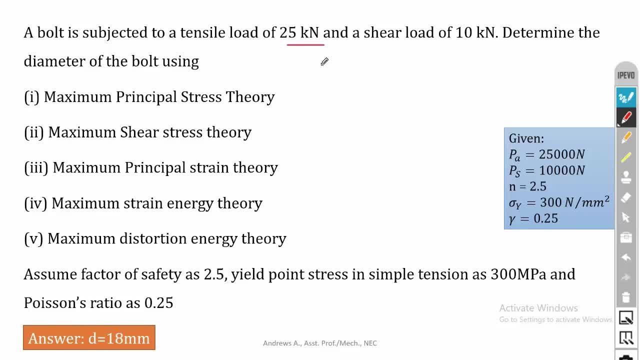 is subjected to a tensile load of 25 kN and a shear load of 10 kN. So the problem is almost same. Determine the diameter of the bolt using maximum principle stress theory, maximum shear stress theory, maximum principle strain theory, maximum strain energy theory, maximum distortion. 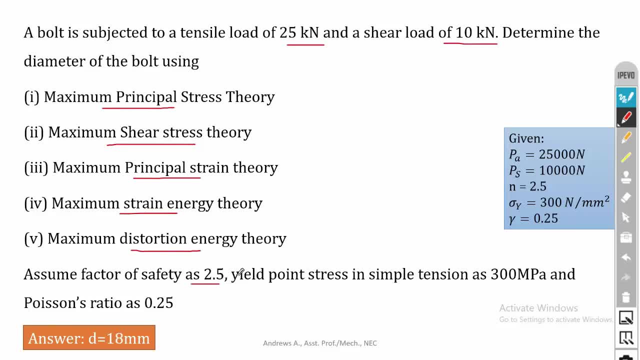 energy theory. Assume factor of safety as 2.5. So here in this problem n value is given, So n is equal to 2.5. So we have to substitute the value of n in our theories of Euler equation. Then the yield point stress is given, that is 300 MPa. So sigma y is 300 N per mm. square. 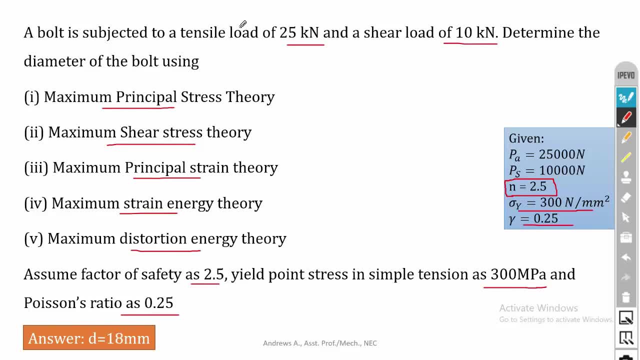 and the gamma is given, it is 0.25.. So the axial load is 25000 and the direct shear load is 10000.. So first we have to calculate the sigma a and tau, Then from sigma a and tau we have to calculate. 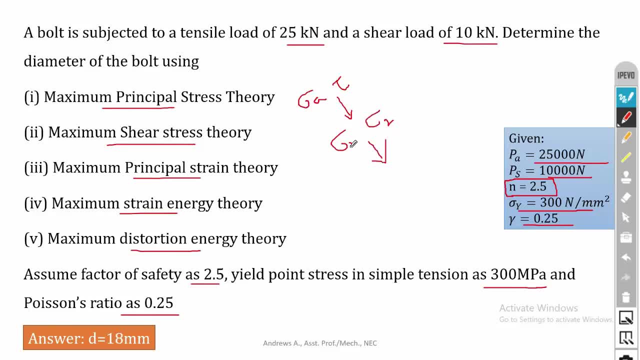 sigma 1 and sigma 2.. Then from by using this sigma 1 and sigma 2 in theories of Euler equation. finally, we have to calculate the value of diameter using all the theories.